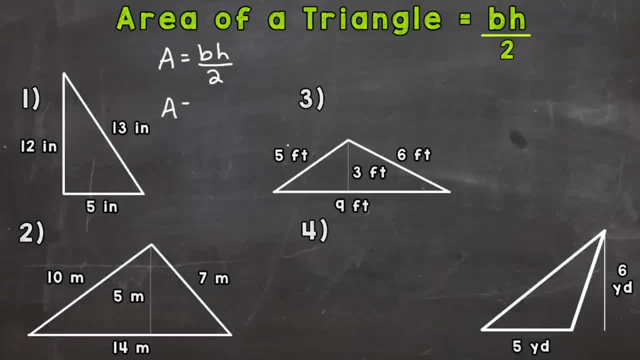 height. So now under our formula, we're going to plug in our base and height. so our base of 5 inches down here, this is the base of our triangle. So 5 times the height, right that 12 inches. So I plug in the 12 and we divide that by 2. 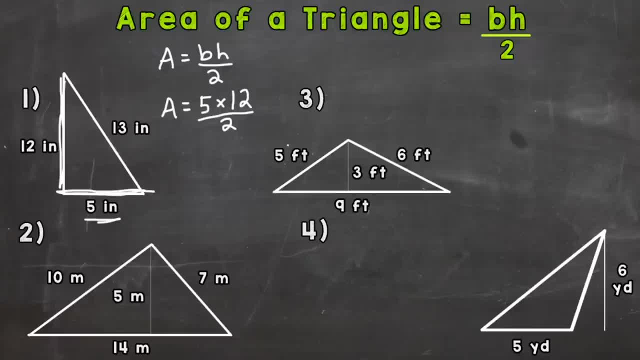 and I'll tell you why at the end of this problem, why we divide by 2.. So now it's time to solve. So we know, 5 times 12 is 60 and now we need to do 60 divided by 2 to get to our answer and notice we have 60. 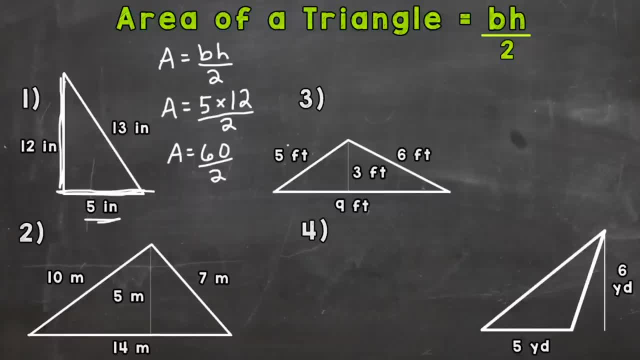 divided by 2, written as a fraction there. That's fine. a fraction is division, So that just means 60 divided by 2, which gets us to 30.. Now we need to put our unit of measure, which is inches, and we put a 2 up here and we read that as area. 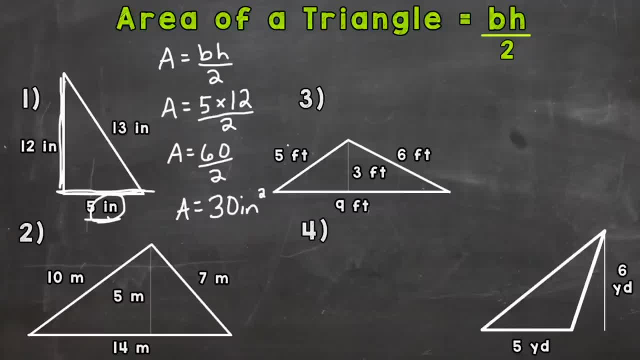 equals 30 square inches And we make that a square unit because there are square inches that cover that triangle, to show how much space that figure takes up. So area equals 30 square inches. Now let's go back to why we divide by 2. So we have a triangle here. 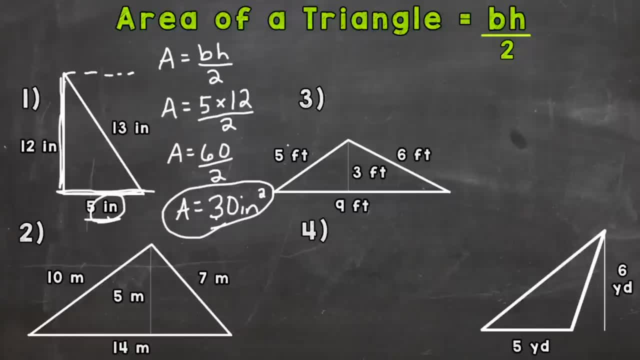 I'm going to draw some imaginary lines to make this a rectangle, slash, parallel a gram. So in order to find the area of that parallelogram or rectangle, we would do 5 times 12, the base times the height, or length times width, and that would get. 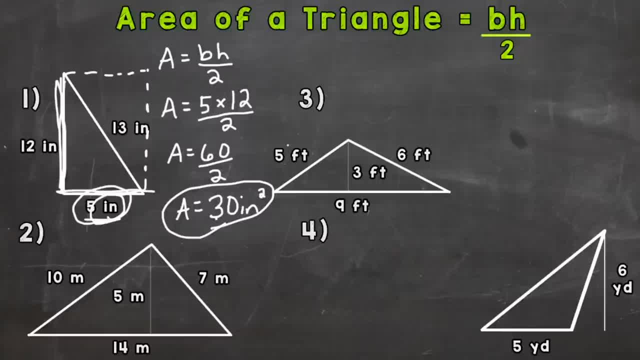 us 60. But this triangle is exactly half of that rectangle or half of that parallelogram. So we divide by 2 to give us the area of the triangle or half of that rectangle or parallelogram. So let's go to number 2 here And we start by writing out our formula: Area. 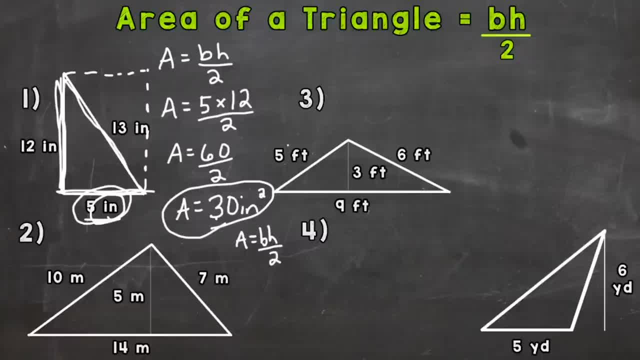 equals base times height divided by 2.. Now we plug in: Area equals base is 14 meters here times the height of 5 meters. We do not need the 10 or the 7. And then we need to divide by 2.. So area equals. well, 14 times 5 is 70. And we need 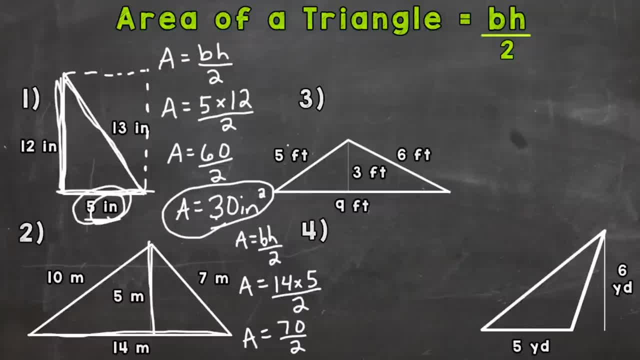 to divide 70 by 2 to get our area. So area equals 35 meters squared. And again we use square units because there are 35 square meters, 1 by 1 meter squares that we need to divide by 2 to get our area. So area equals base times height divided by 2.. 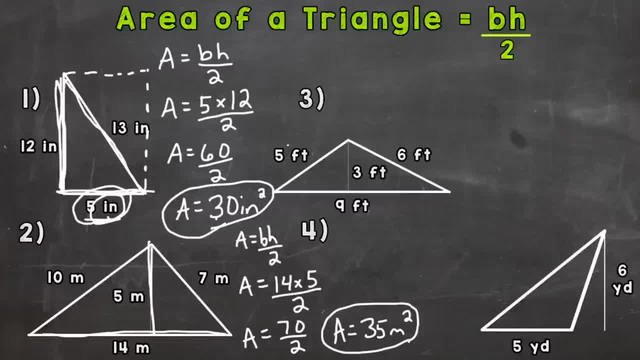 So for number 3, let's start by writing out our formula. It's always good habit just to start by writing out the formula. So we have area equals base times, height divided by 2.. Now hopefully we know that we plug in next. So base right here, the base of the triangle. 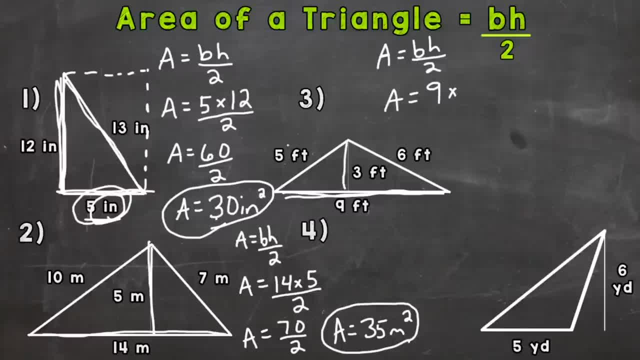 is 9 times the height. How tall is that triangle 3.. And then we plug in: Area equals base times height divided by 2.. And then we plug in: Area equals base times height divided by 2.. And then we plug in: 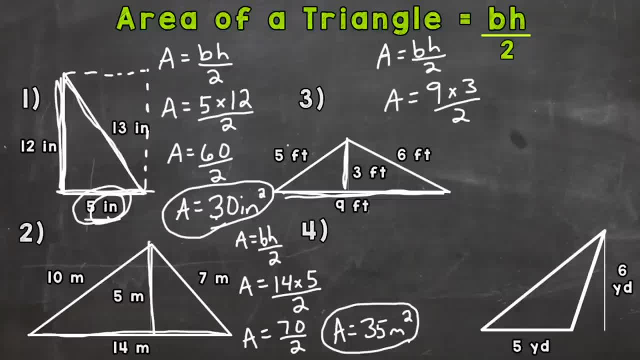 3 feet And we divide that by 2.. So we get 9 times 3 is 27 divided by 2.. So our area- and this one's actually going to give us a decimal- 13,5 or 13 and 5 tenths square feet. 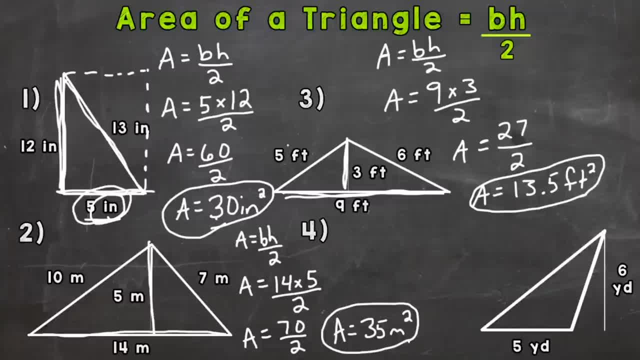 And lastly number 4 here. So we start with the formula: Area equals 3.. We have 9 times equals, base times, height divided by 2. now we need to plug in. so our base down here is 5 yards and we multiply it by our height. now our height is outside the.